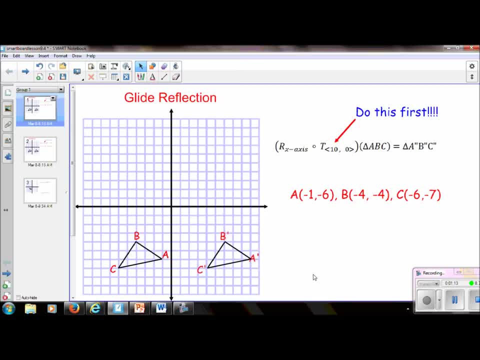 the next thing that I need to do is do the reflection over the x-axis. So if I were to reflect this triangle here, I would end up right here And just to review: when I do reflection, I always need to be the same distance. 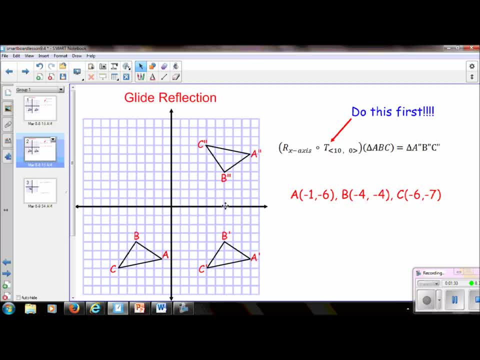 So this is 4 units this way, it's also 4 units this way. So, from A prime to the line of reflection at 6, and then to A double prime, it's 6.. So that is a perfect example of a glide reflection. 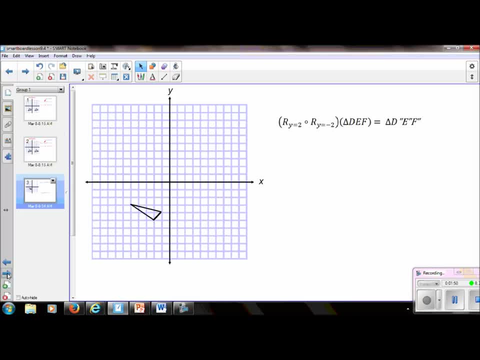 We're going to do one more composition. This one is a double reflection And remember that we have to start here first. So we need to do this reflection. And I didn't label this triangle with the letters because I actually felt like visually it was just. 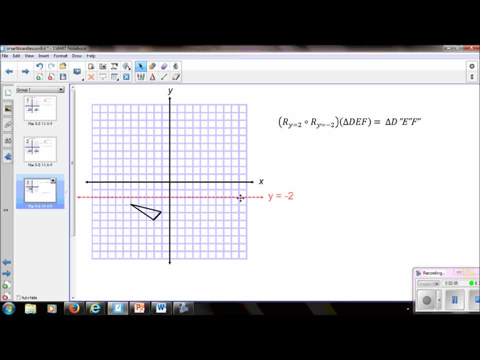 too much to look at with all these letters with multiple reflections. so the first reflection is from the line of reflection y equals negative 2, which I have listed here. so again, this is crossing the X, I mean the y-axis, at negative 2, and then if I were to reflect that, it would end up right here now. I. 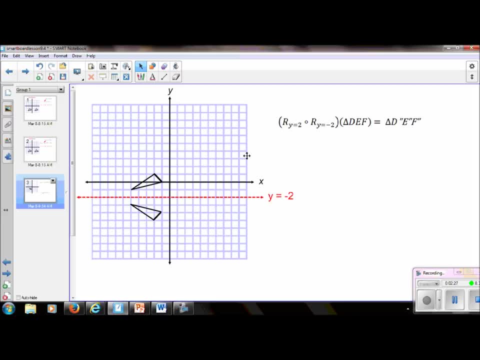 need to do the second reflection. this has a line of reflection of y equals 2, so this time it's crossing the y-axis at positive 2 and it is a horizontal line. so now, if I were to take this shape that I've just reflected and reflect it again, 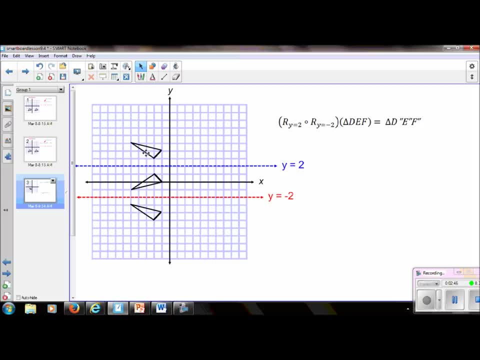 it would end up right here now. what I want you to do is take a look at our pre image and where we ended up. they are just a translation. so when we do a double reflection, or a composition of reflections across two parallel lines, it ends up just being a translation. so 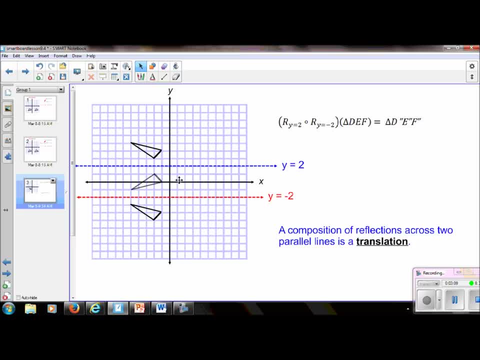 let's actually just take this out of here, rats, I can't take it out of there. we go and then look at these two, so when we've moved out that middle reflection, you can clearly see. it's just a translation. we could have used this notation to do the same thing that we did right here. a.